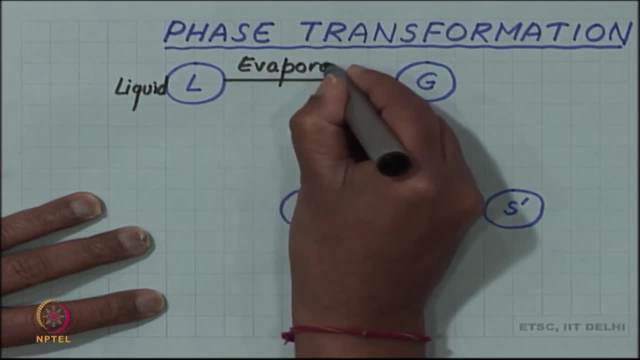 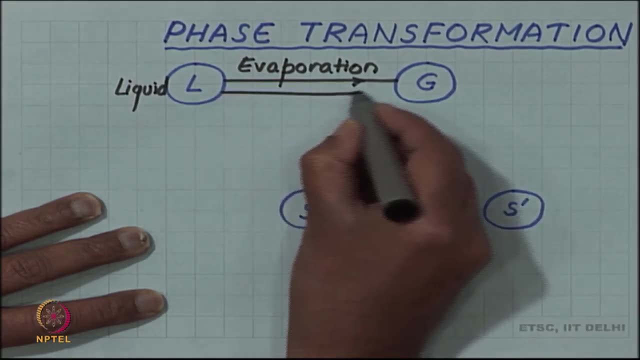 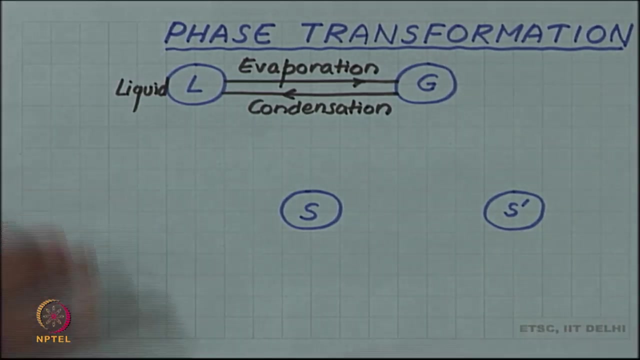 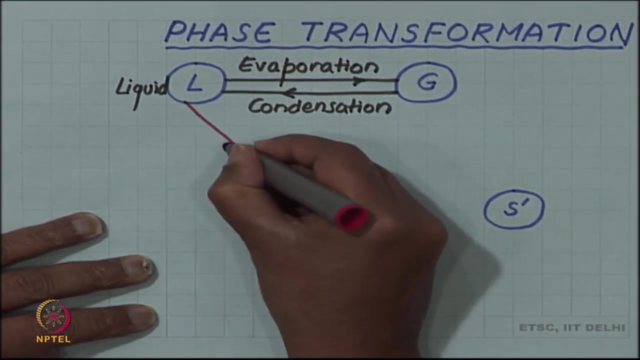 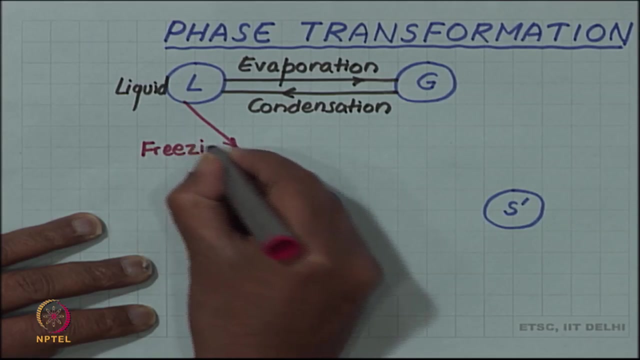 of evaporation. The gas can also condense back into liquid, So we have condensation. A liquid can freeze into a solid, So we have freezing. Or a solid can melt, So we have a condensation, So we have a condensation, So we have a condensation. 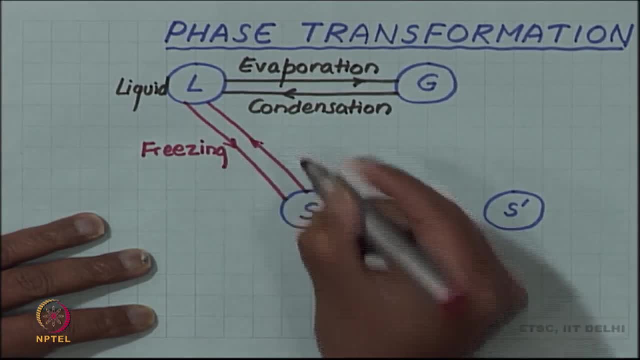 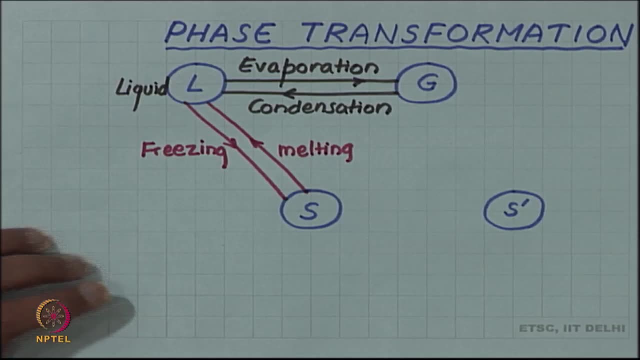 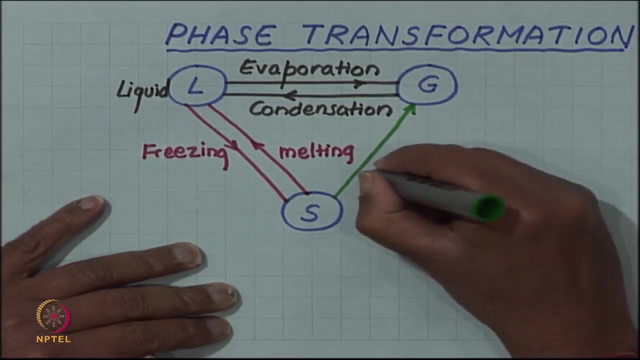 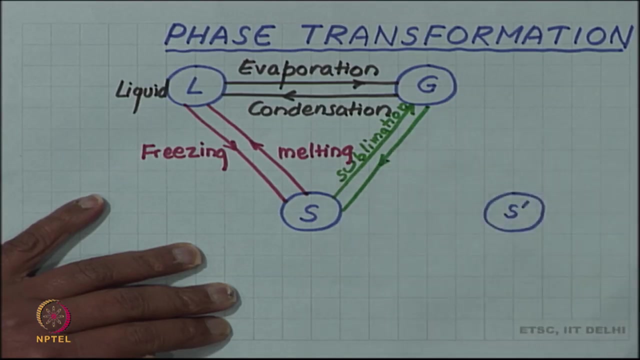 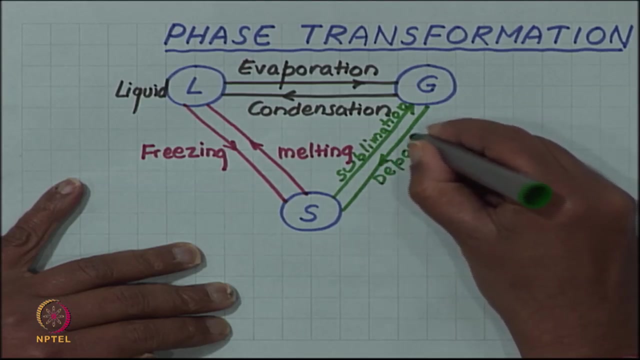 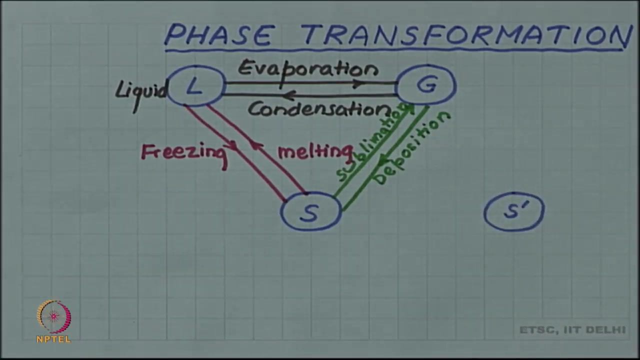 A solid can directly sublimate into liquid. We have melting. A solid can directly sublimate into gas, A process called sublimation- Or a gas can condense back into solid- We can call this deposition. And a very important class of transformation is one in which one solid phase transforms. 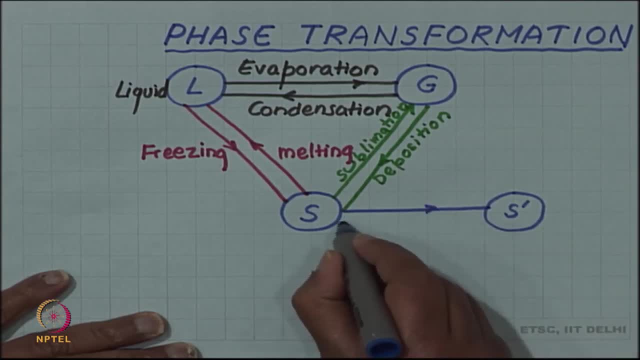 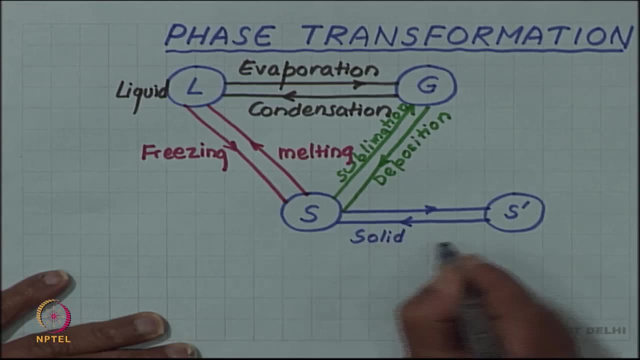 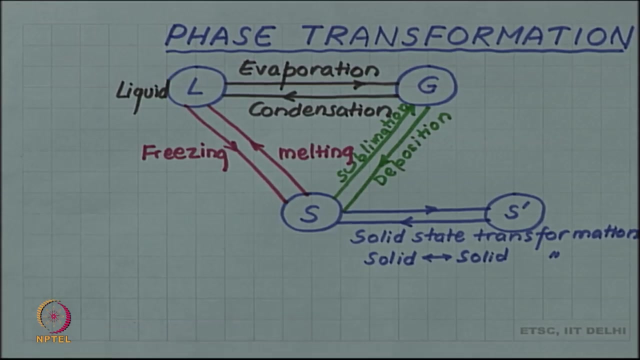 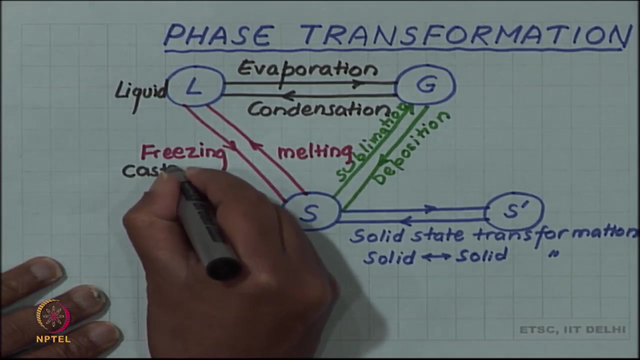 into another solid phase, So we can have a solid-solid transformation, Solid state transformation, Sometimes known as solid-solid transformation. Some of these transformations are technologically very important. So, for example, freezing is used in casting, So Test mission is used in casting. 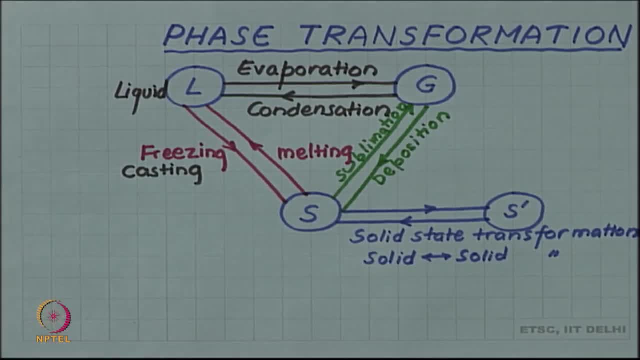 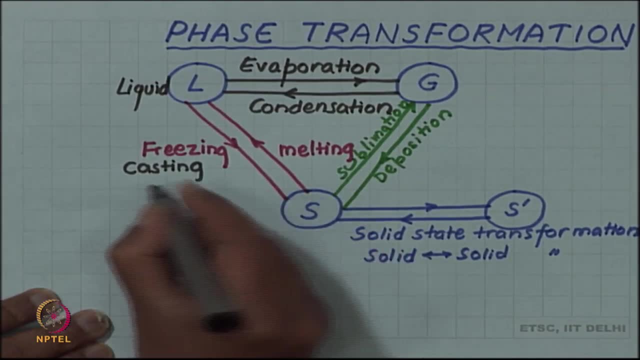 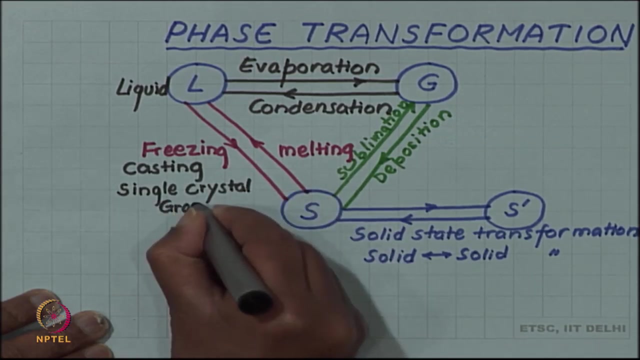 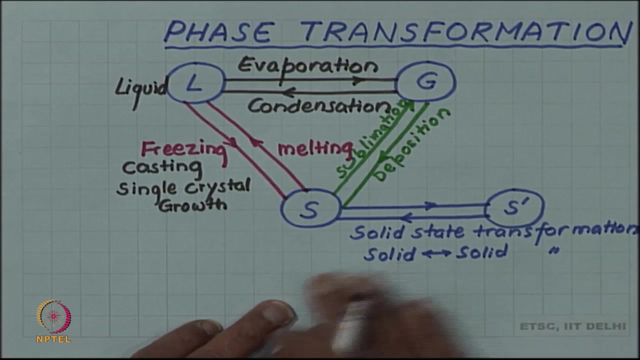 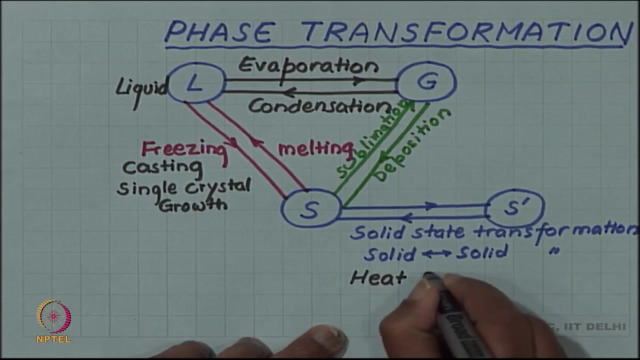 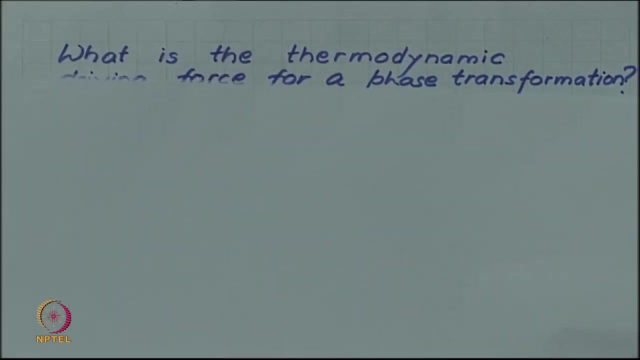 Which is a very important engineering process for fabricating many components. You also in the modern semiconductor industry there is a single crystal growth and solid-solid transformation we will see is used very much in a process called heat treatment. Let us now look at the question that what is the driving force? the thermodynamic driving. 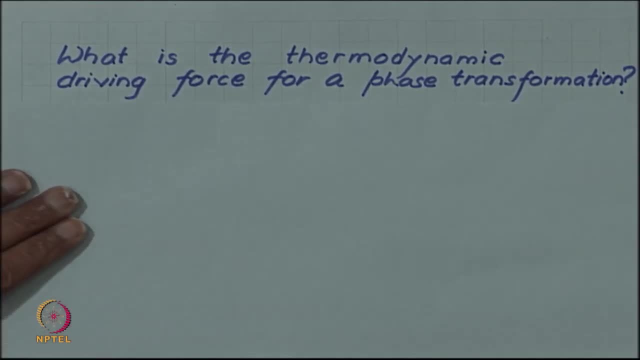 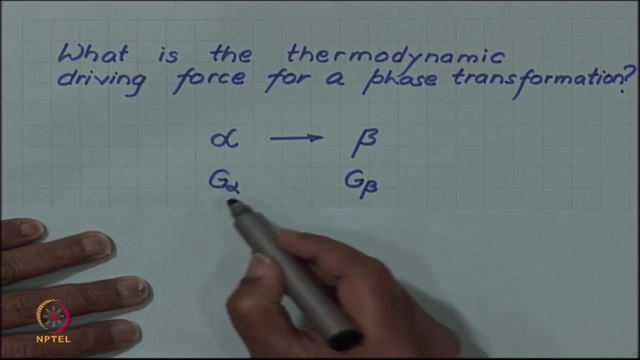 force of a phase transformation. By driving force we mean that when a phase alpha is transforming into beta, Then the free energy of the two phases will be different. So the alpha phase has a free energy- G alpha- whereas the beta phase has a free energy. 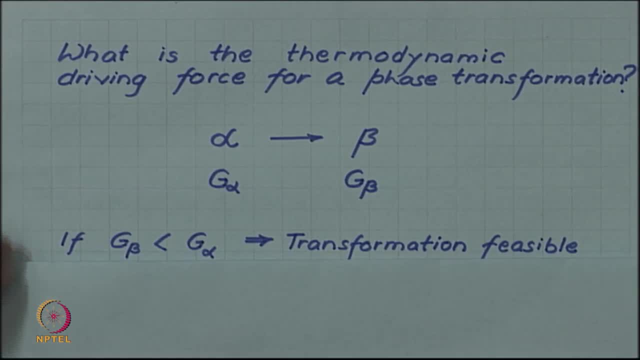 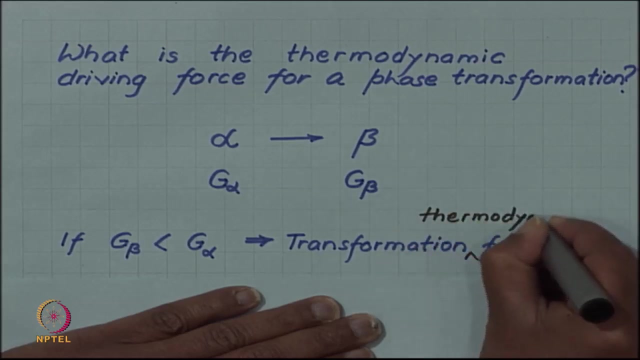 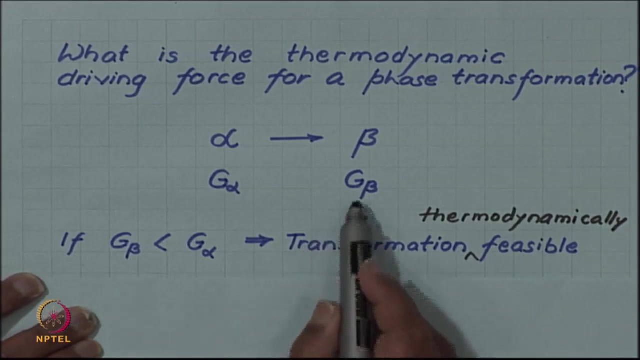 G beta. The difference between these two phases control the phase transformation. The phase transformation will be thermodynamically feasible. so the transformation is thermodynamically feasible Only if the final product phase G beta has a lower free energy than the starting phase alpha. 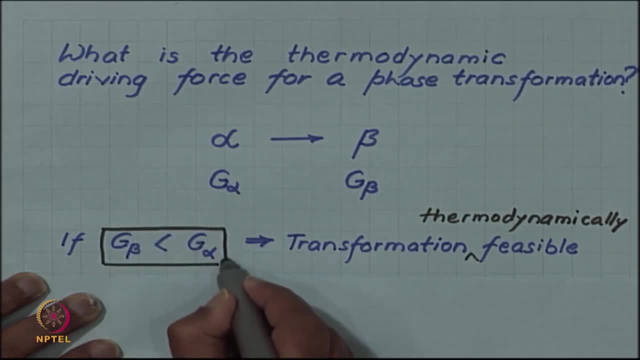 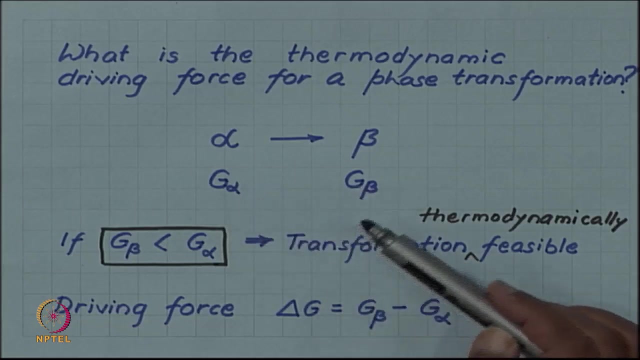 This is an important condition for phase transformation to occur at constant temperature and pressure. So this difference. So since beta has to have low free energy, So since beta has to have low free energy, So since beta has to have lower free energy than alpha for transformation to happen, lower, 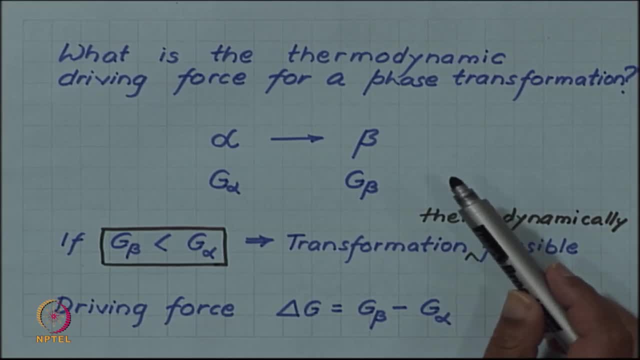 is G beta in comparison to G alpha, higher is the driving force. This is what we mean by the driving force. So the driving force is the difference between the free energy of the two phases. This difference is what we call the driving force. 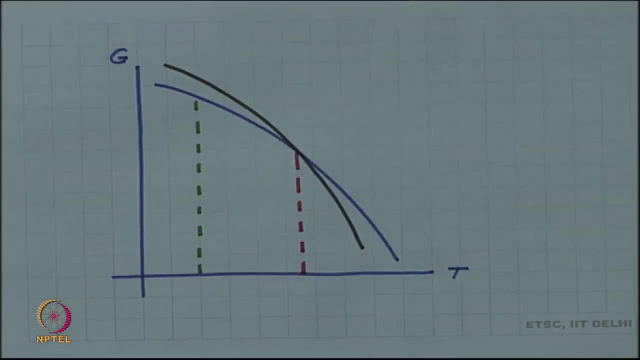 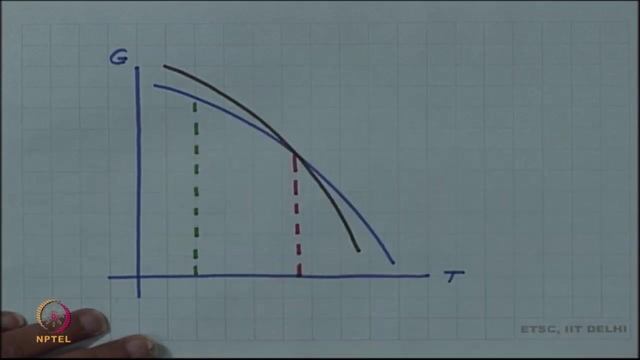 Okay, Let us look at what the free energy curves look like. So here I have drawn free energy as a function of temperature for two different phases. So the one phase shown in black, let us say, represents the liquid phase, whereas the other, 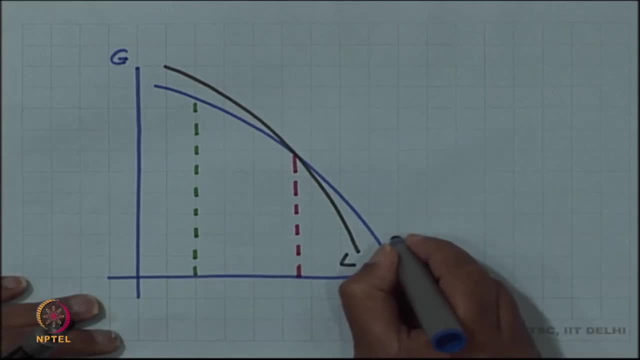 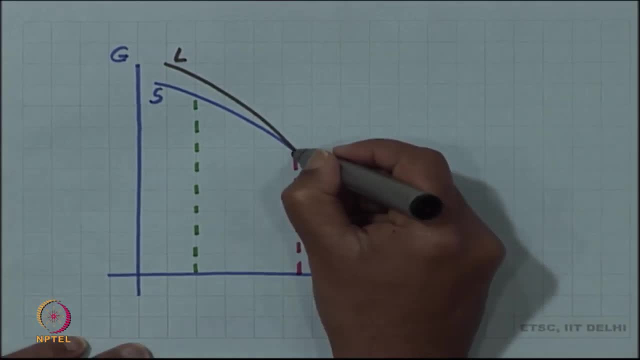 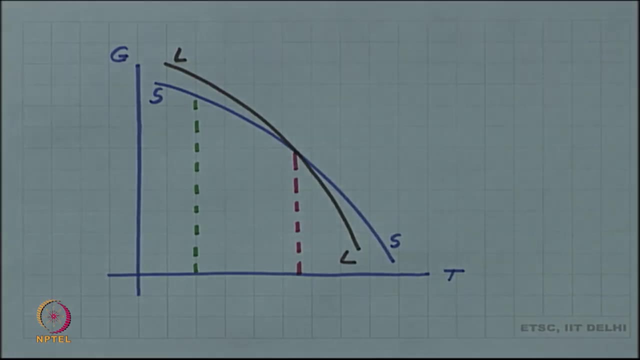 You can see that the two free energy curves are intersecting at a given temperature. So at that temperature the two phases have the same free energies. So this is the temperature which is called the thermodynamic melting point. So at the melting point, 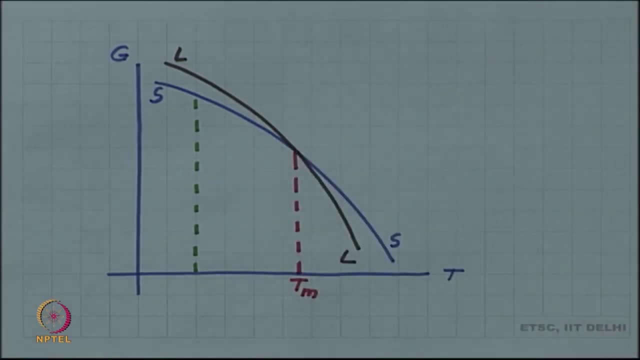 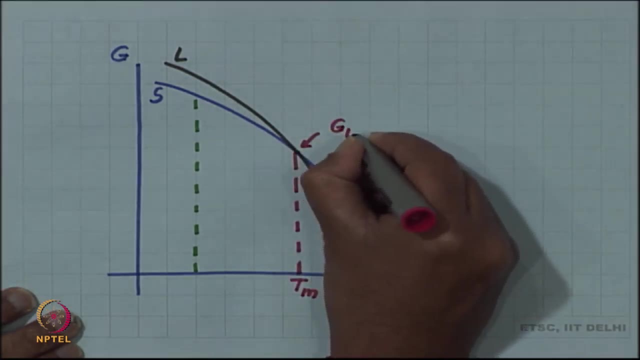 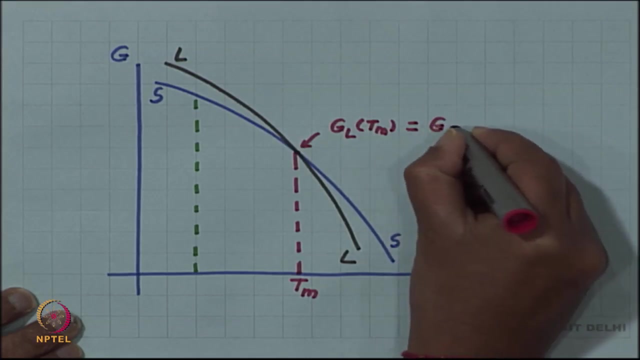 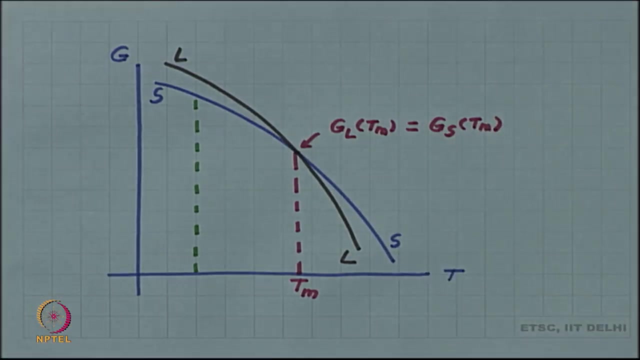 So the two free energy, g alpha and g beta, are equal. free energy of the liquid phase at the melting point is same as free energy of the solid phase at the melting point Below the melting point. So below the melting point One can see that 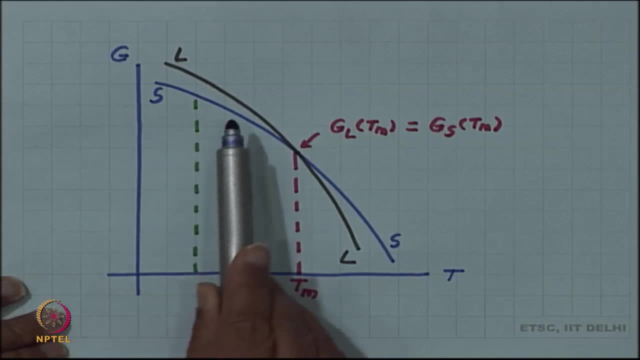 Okay, So the solid phase has a lower free energy than liquid phase, So liquid can transform into solid below the melting point, whereas solid will melt into liquid above the melting point. So if we have some transformation temperature represented by this green vertical T, then 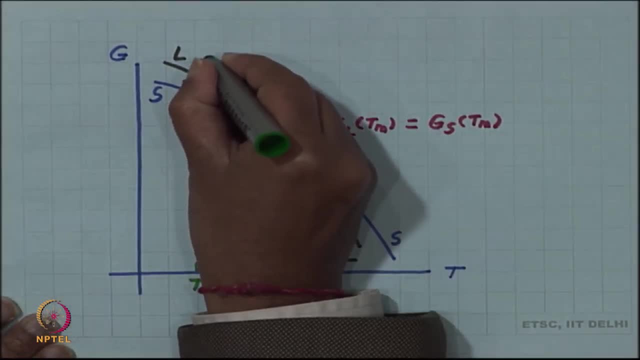 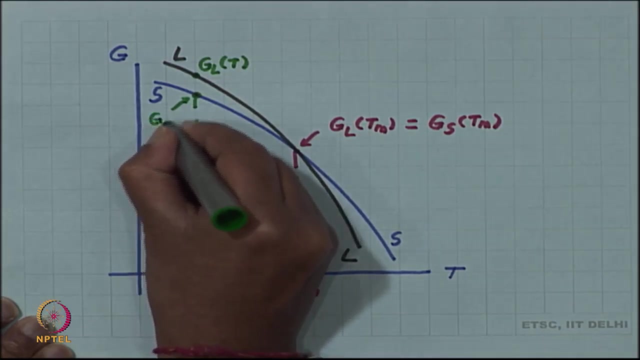 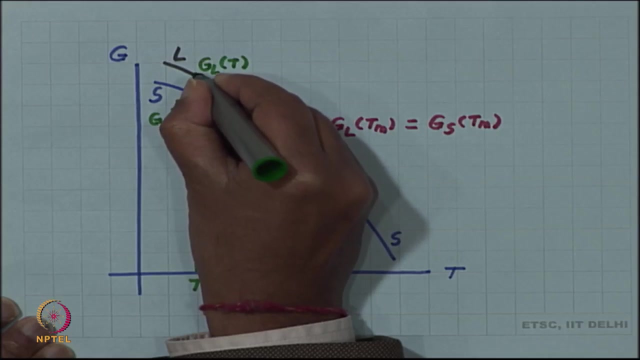 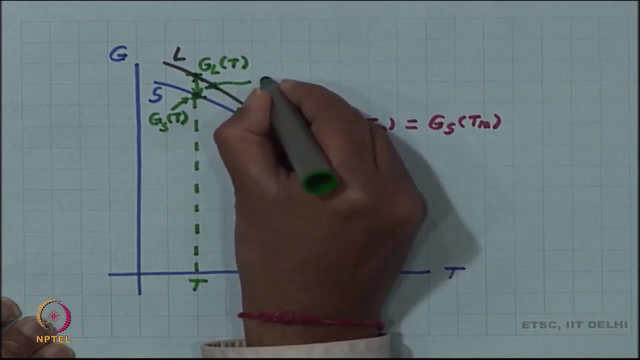 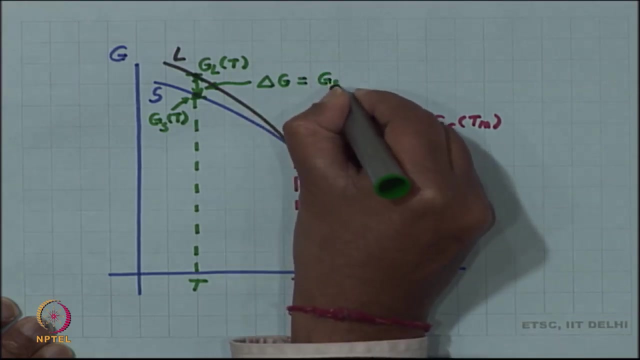 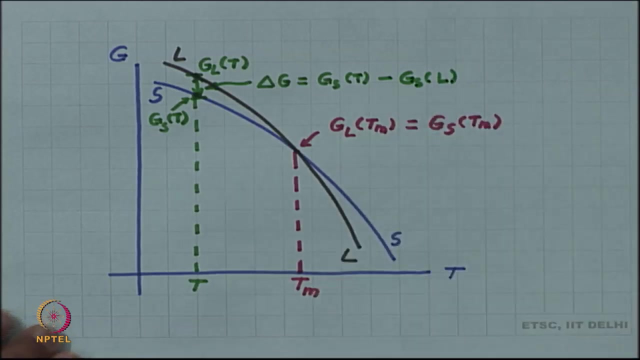 at that transformation temperature, the liquid phase has a higher free energy- Okay- Whereas the solid phase has a lower free energy. So the difference between the two phases, this difference is what will be the driving force. Okay, So delta, G, g s T, minus g s L. 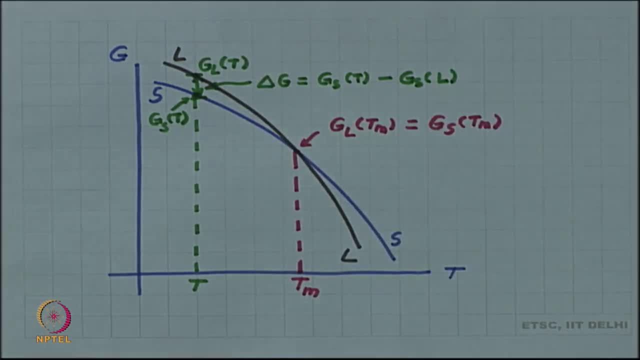 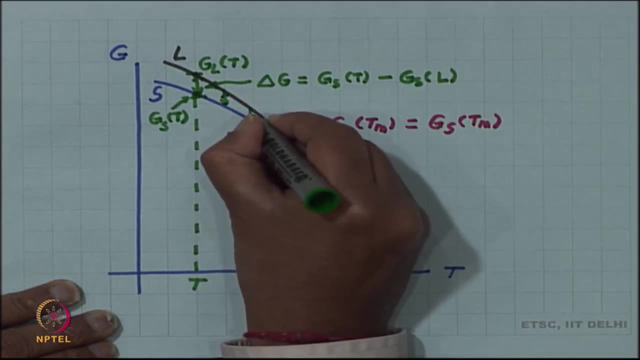 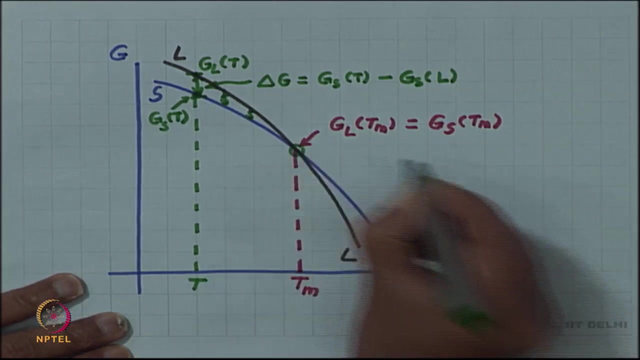 We can see that this driving force is actually a function of temperature. So if T was closer to the melting point, its value, the driving force value, will be lower. And exactly at the melting point the driving force is actually 0.. Okay, Delta G, because the two free energies are the same. the driving force is 0 at the thermodynamic. melting temperature. So that is why, for actual freezing to happen, some amount of under cooling is essential. Let us now have an estimate of the in this free energy difference, or the driving force for freezing. So by definition, this driving force is free energy of solid minus the free energy of liquid. 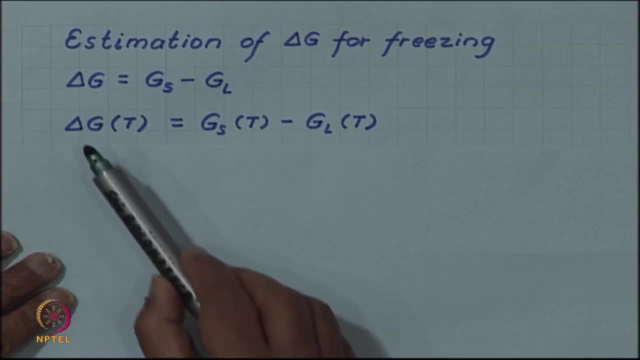 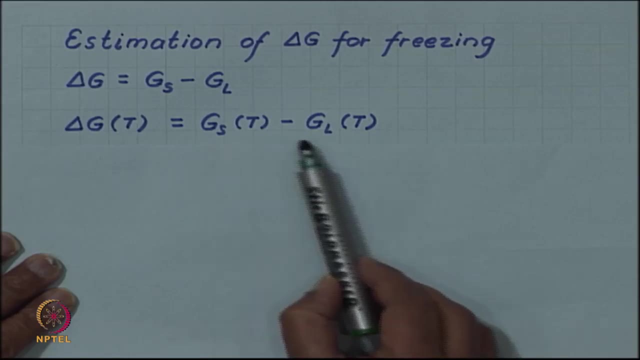 Since all these quantities are functions of temperature, we write them as delta. G as a function of temperature, T is equal to g. s as a function of temperature, minus g L as a function of temperature. Now, if we evaluate this at the melting point, Okay, 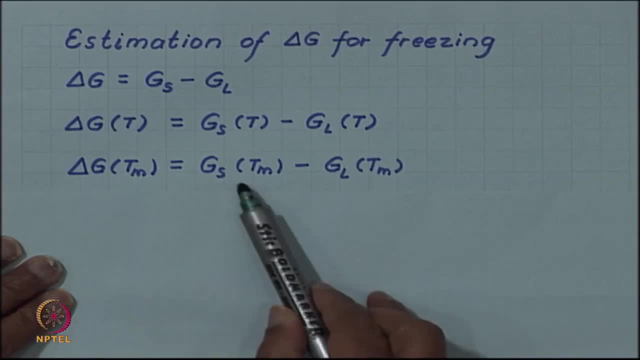 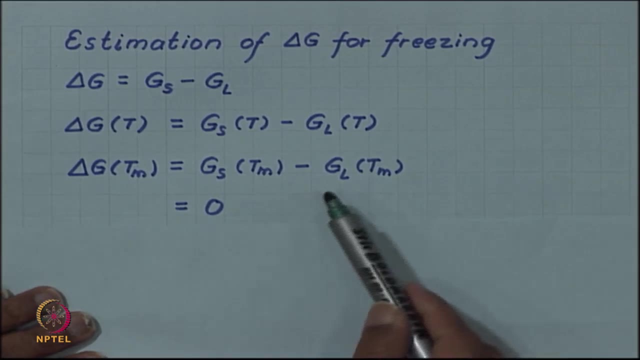 Then we have an expression Like: delta G T m is equal to g s T m minus g L T m. But we have seen that g s and g L are equal at the melting point. So this free energy difference, delta G T m, is 0.. 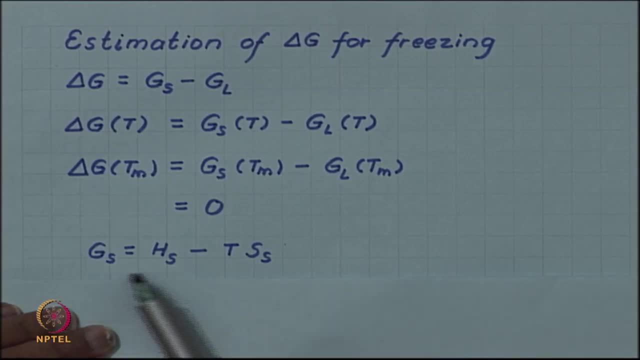 Now, at any given temperature, we can write as: g s is equal to h s minus T s and similarly, g L is equal to h L minus T m. Okay, Okay, So delta G T m is equal to g s L. If we take the difference, then the difference is the free energy change delta G, which will 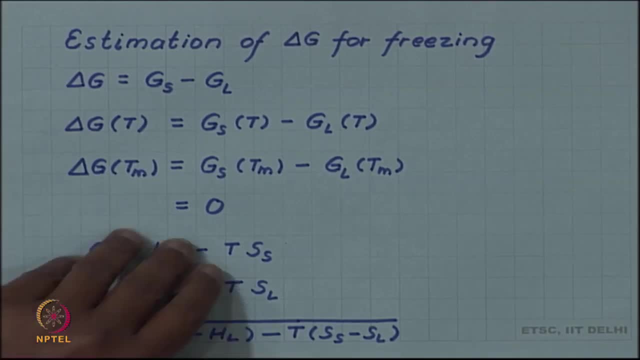 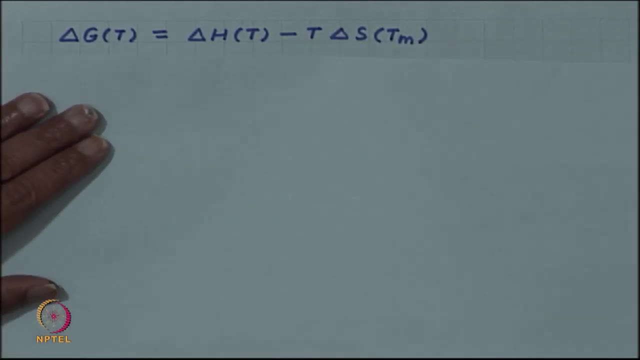 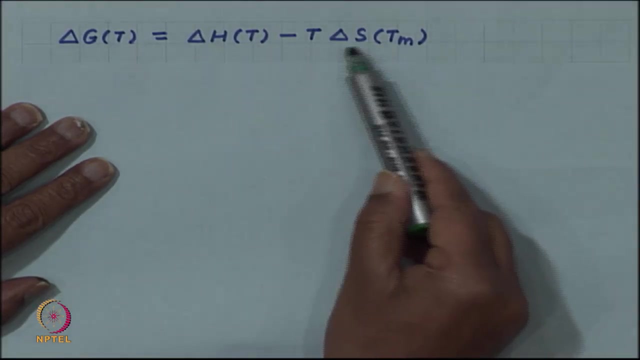 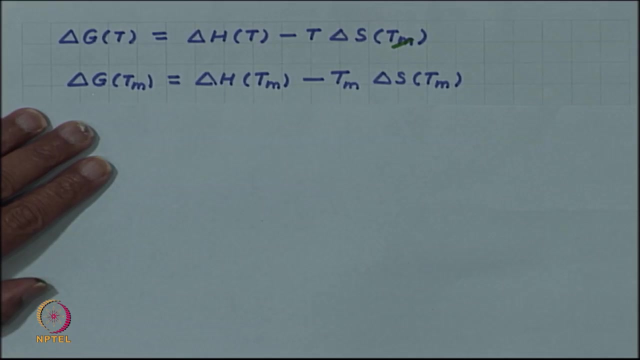 be h s minus h L minus T times s s minus s L. So this we can write as delta H evaluated at T minus T times delta S evaluated at T. Okay, If we evaluate these quantities at the melting point, then we have delta G. T, m is equal to. 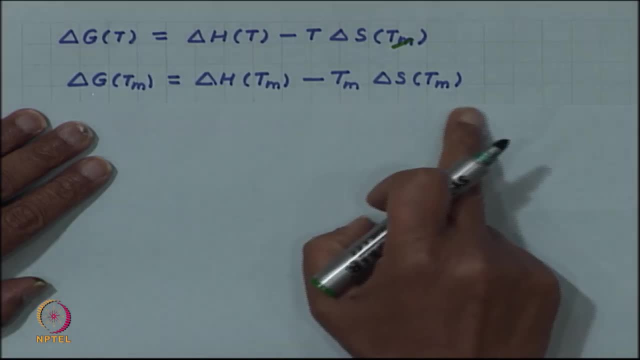 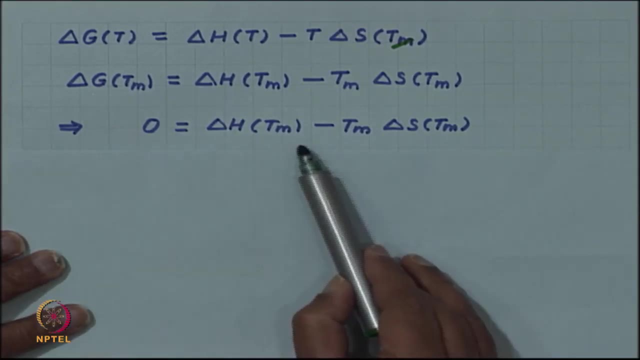 delta H T m minus T m. delta s T m. But we have seen delta G T m is 0. So we can write: 0 is equal to delta H T m minus T delta s T m. So if we rearrange. 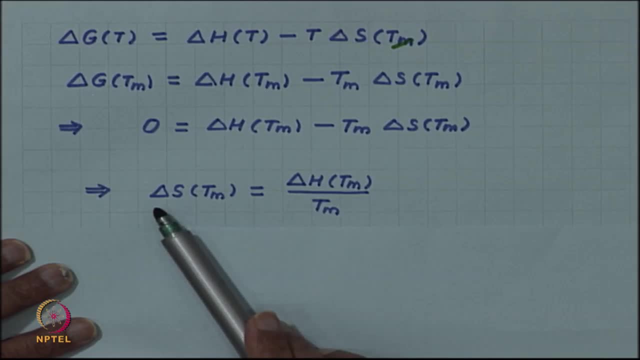 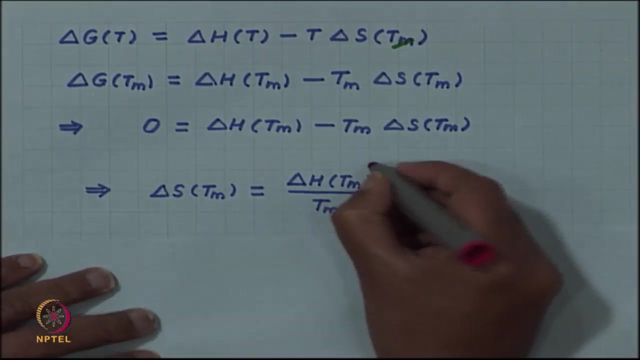 We see that. Okay. So the heat of melting, the entropy change upon the transformation, upon freezing, at the melting point, is nothing but enthalpy of melting divided by T- m. and this enthalpy of melting is nothing but what we commonly call as latent heat of melting. 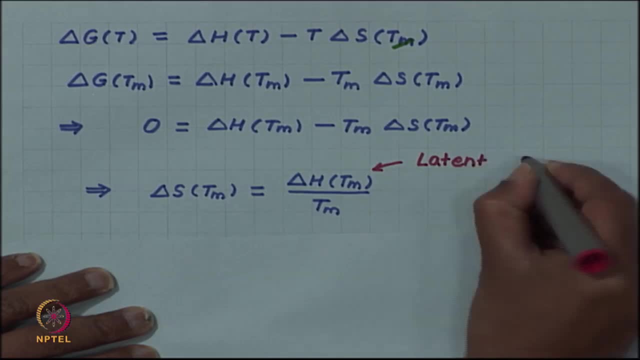 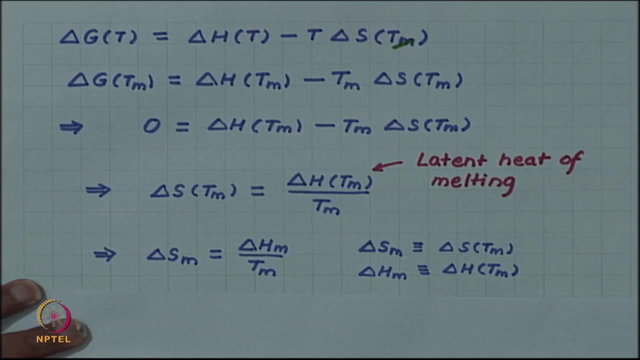 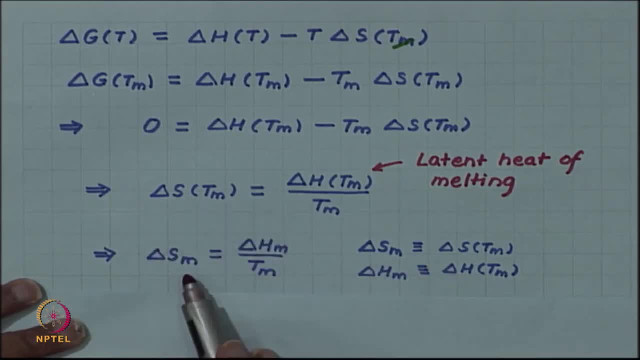 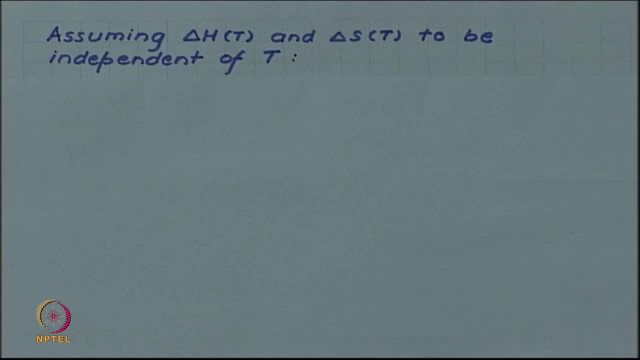 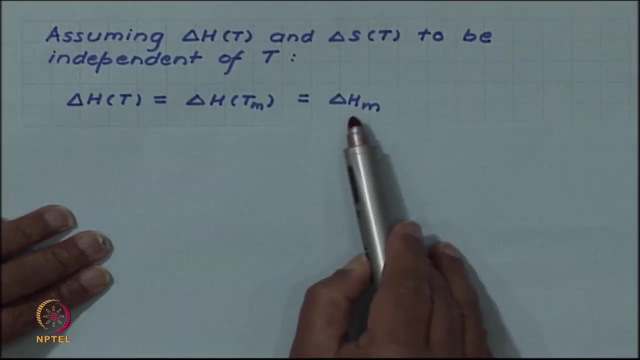 is vimiform. But if we translate by assuming that the result of delta H and delta S in the range among this is log n is v, they are not varying rapidly and effectively. they are independent. If we make this assumption, we can assign the value of delta h t equal to that at the freezing temperature. delta. 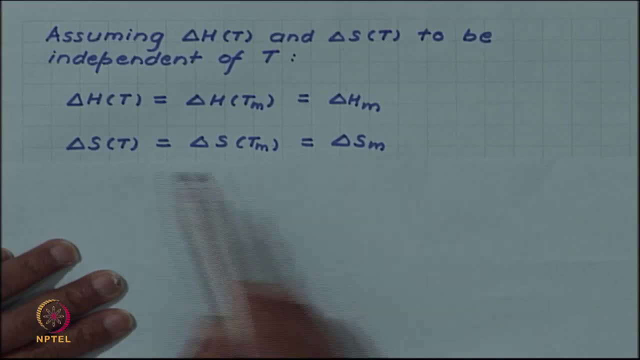 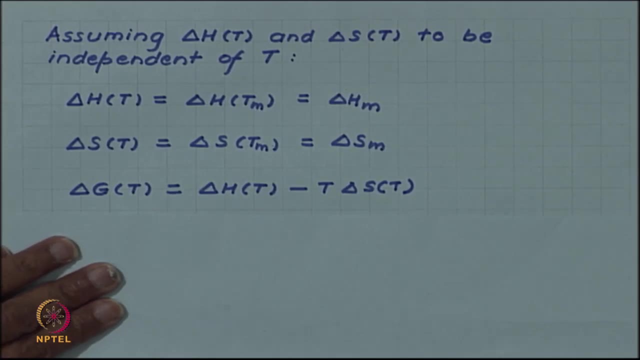 h m and similarly delta s m can be assigned to delta s t. With this assignment and with this assumption, we can rewrite our free energy difference. delta h t is delta h t minus t, delta s t at simply delta h m. delta h t is now equated to delta h m and delta s t is. 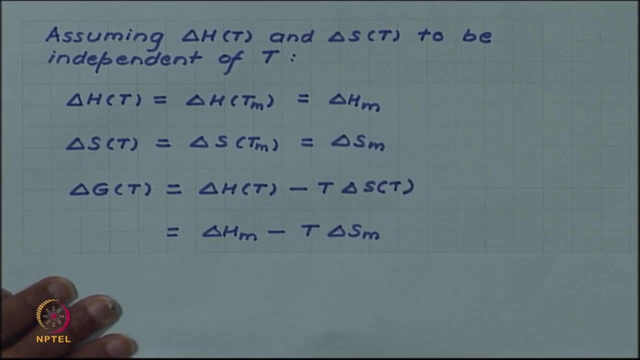 also equated to delta s m. So we have delta h m minus t delta s m. So we have already shown that delta s m is nothing but delta h m minus t delta s m. So delta h m by t m- entropy of freezing or entropy of melting is equal to enthalpy of melting. 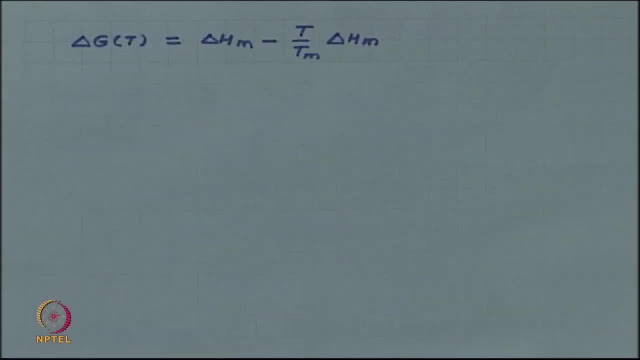 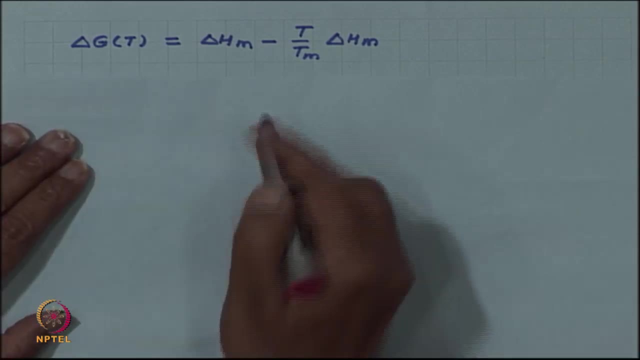 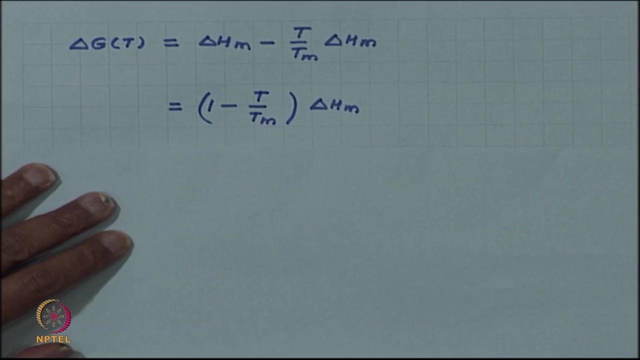 divided by the melting point. So if we now continue with this derivation, we start with this: delta h m minus t. by t m. delta h m, we simply collect the term delta h m. So we have an expression like this, Which we can now write in this way: T m minus t, the difference between the melting point. 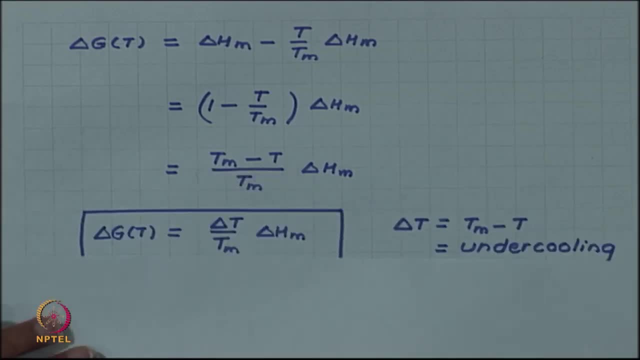 and actual freezing temperature. this is what is called under cooling. So we have write written that as delta t, t m minus t under cooling and we get the expression delta g, t is equal to delta t by t m times delta h m. This is the final expression which is useful. 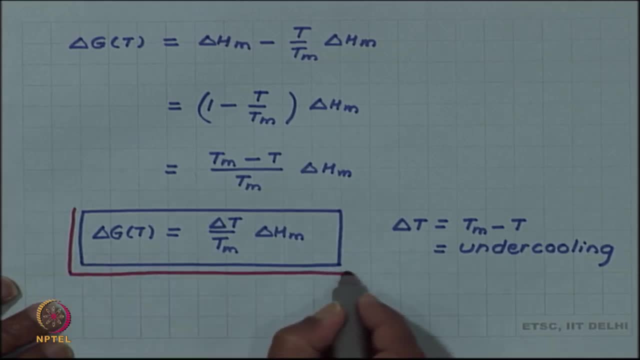 approximation because, See, we we have made certain approximation and the approximation wall, that the enthalpy difference and the entropy difference do not vary as a function of temperature and are constant and their value is equal to their value at the freezing temperature. With this assumption, 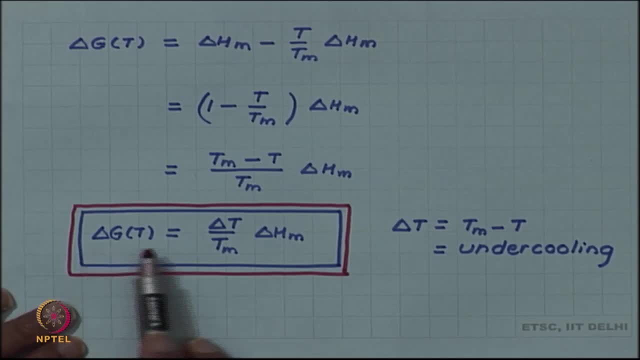 we find that in the free energy change as a function of temperature is linearly dependent upon temperature. more is the under cooling, more is delta, g, t. So this is what we were seeing in the drawing which we had: that more is the under cooling, more is the difference. 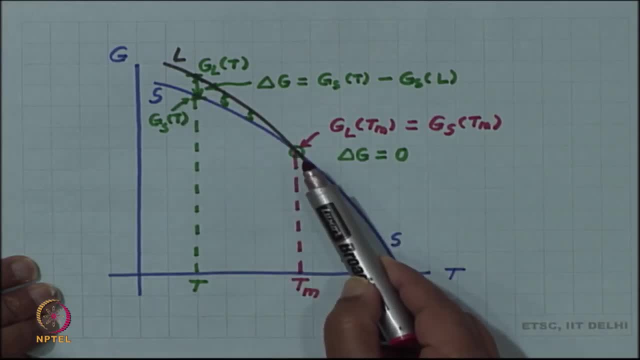 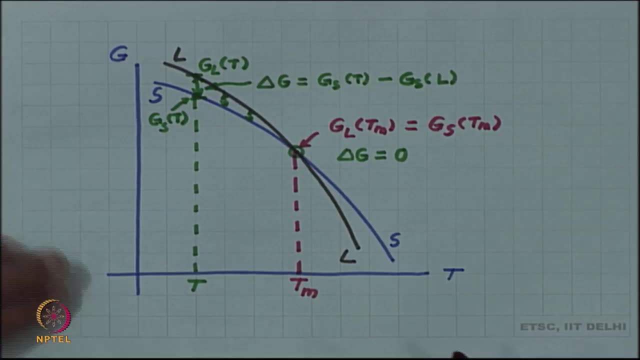 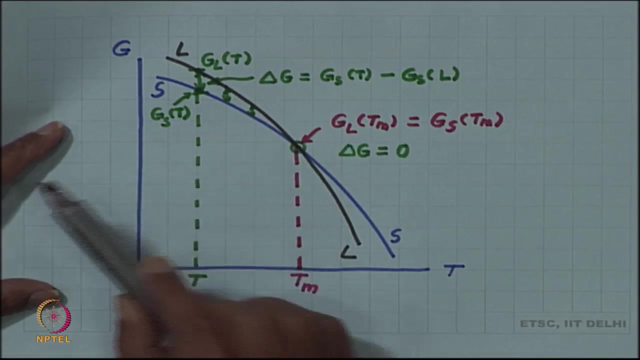 delta g. However, the curve was linear. So essentially our approximation is making these curves as a straight lines. So this is a straight line approximation. So it will be true for certain degree of under cooling, but not very high under cooling. 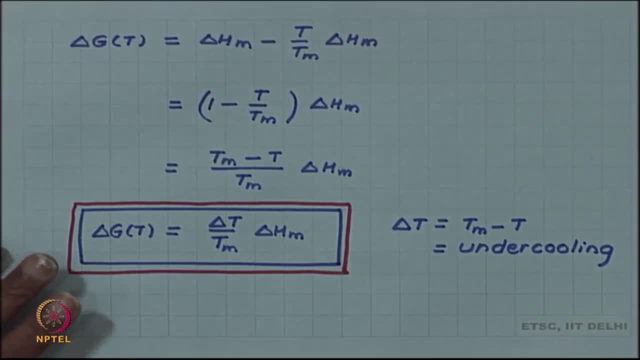 So close to the melting point for small under cooling, we can have this linear approximation for the driving force. So essentially, what we have derived is the driving force for transformation And we have taken as an example- although this will be applicable for any transformation- 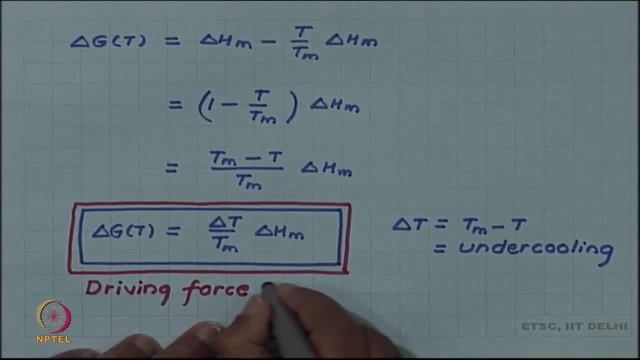 we have taken as an example of freezing, So driving force for freezing, So we have taken as an example- although this will be applicable for any transformation. we have taken as an